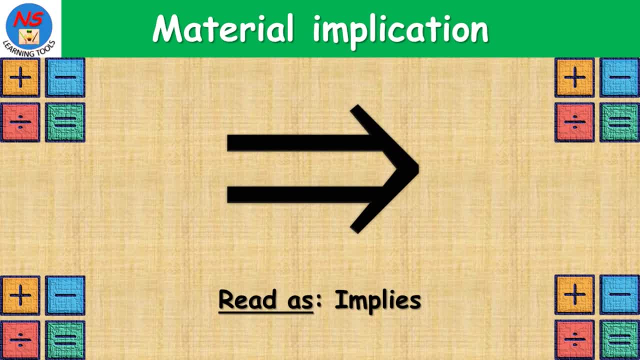 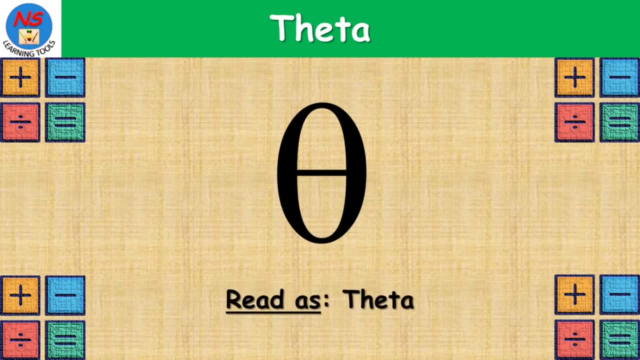 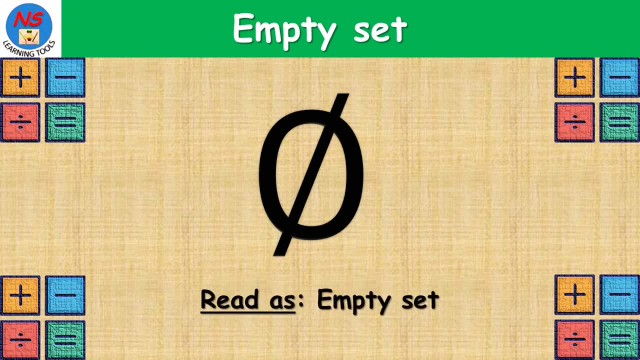 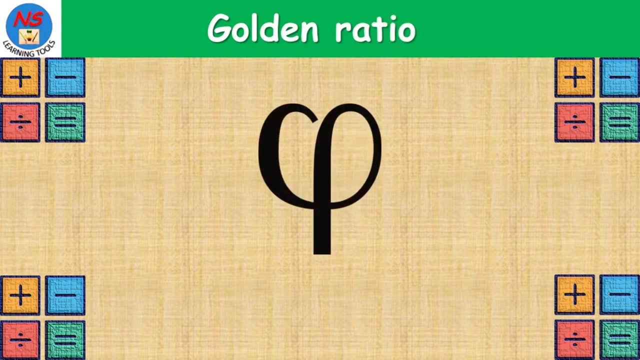 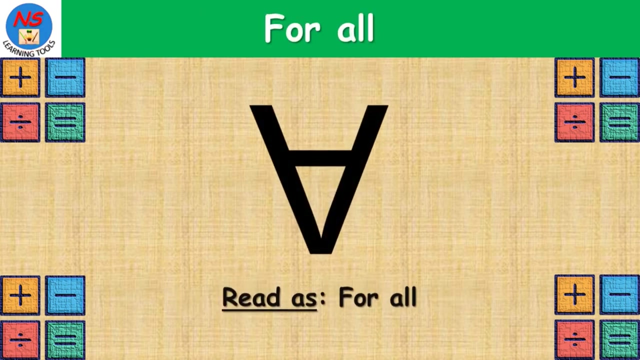 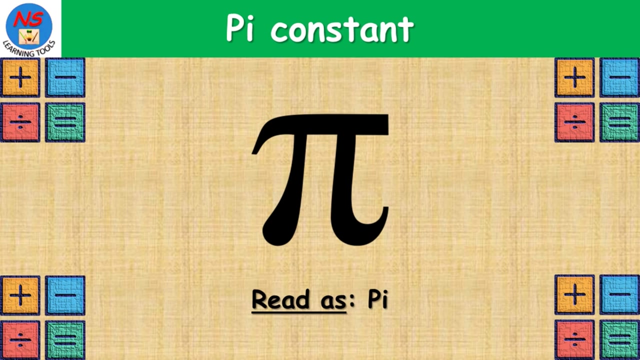 material implication: read as implies or equals. theta: read as theta. empty set: read as empty set. triangle or delta: read as triangle or delta. golden ratio: read as golden ratio. population mean: read as population mean for all- read as for all. pi constant: read as pi. integral: read as integral. intersection: read as intersection of two sets. 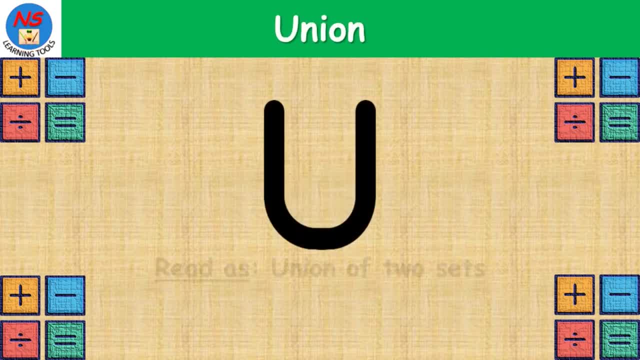 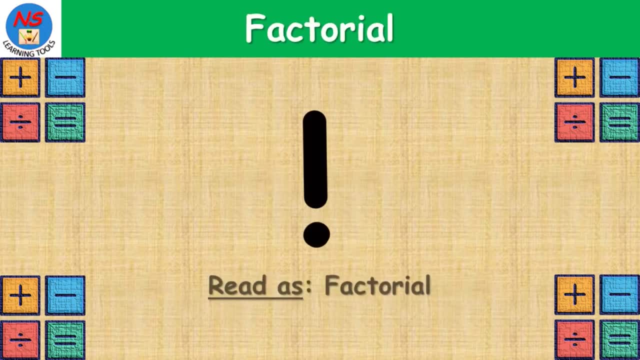 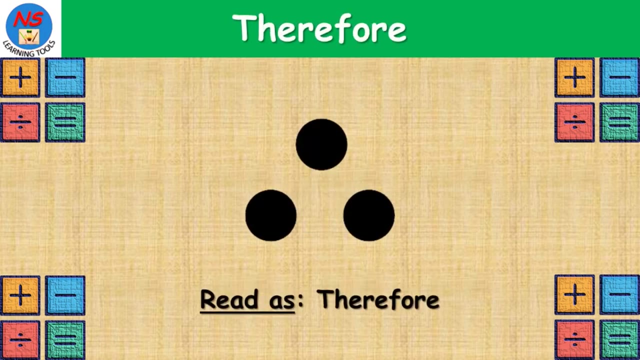 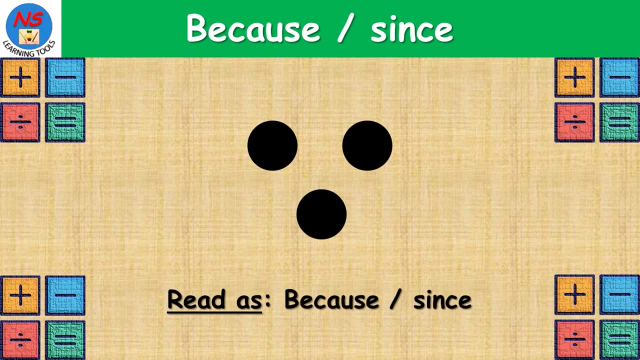 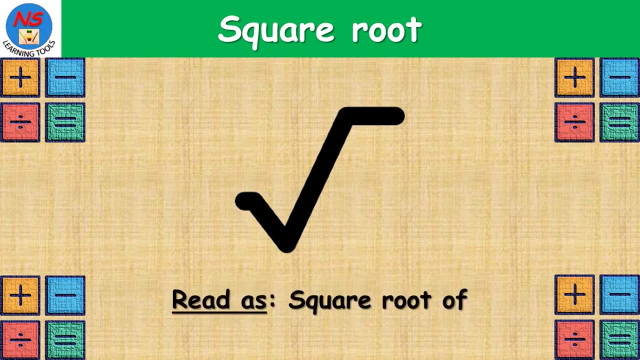 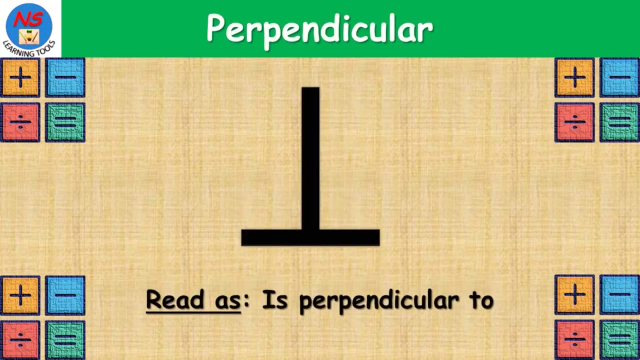 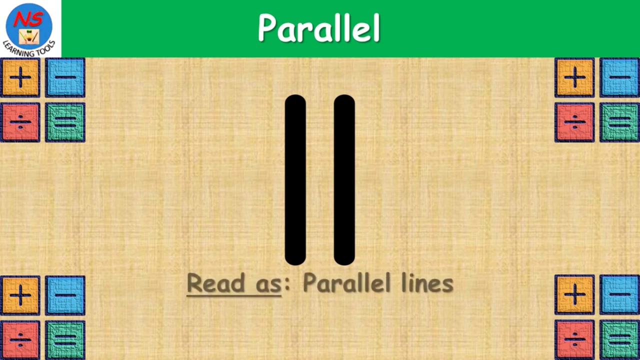 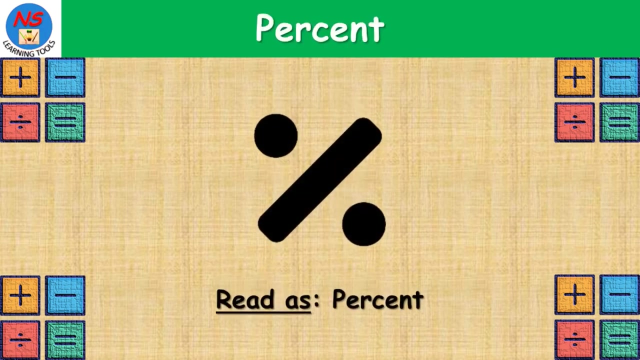 union: read as union of two sets. factorial: read as factorial. therefore, read as. therefore, because or since, read as because or since square root: read as union of two sets- Read as square root of perpendicular. read as is perpendicular to parallel: read as parallel lines exists- read as exists. percent: read as percent. 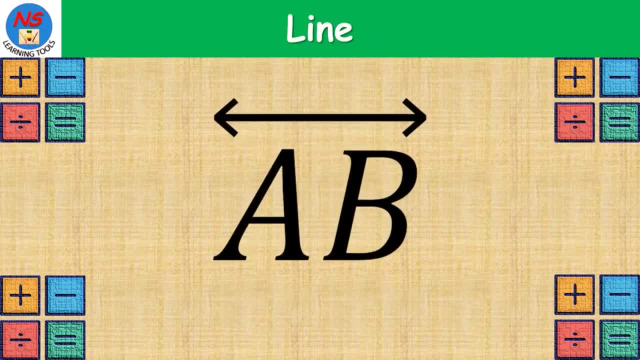 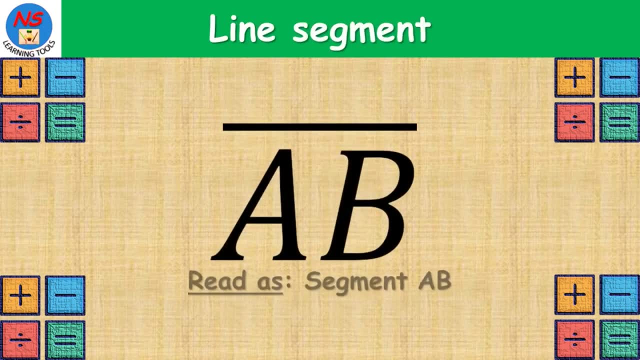 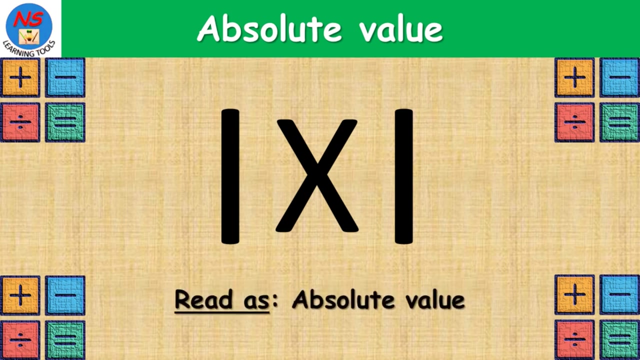 line: read as line a b. line: segment: read as segment a b. ray: read as ray a b. absolute value: read as absolute value. right angle: read as right angle. 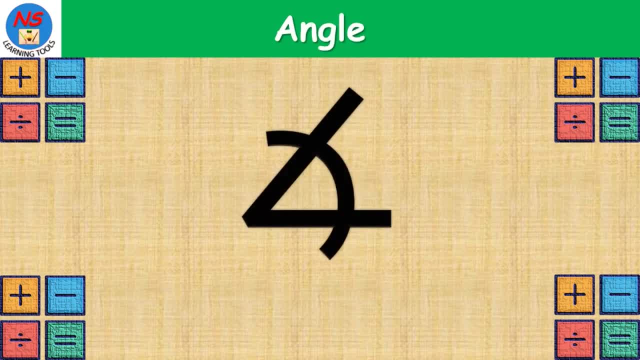 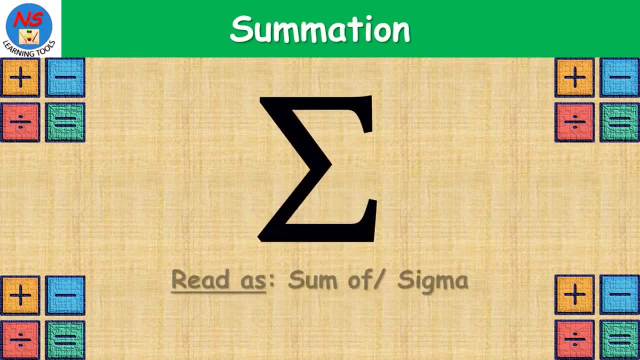 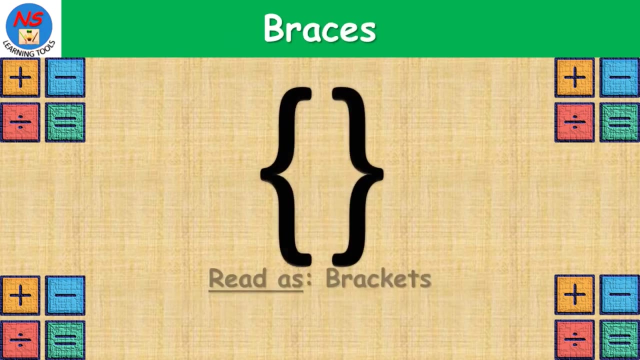 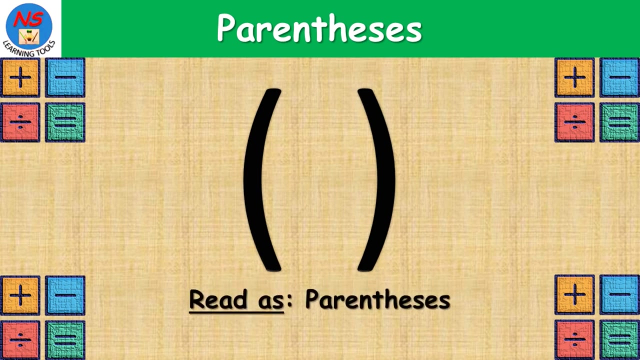 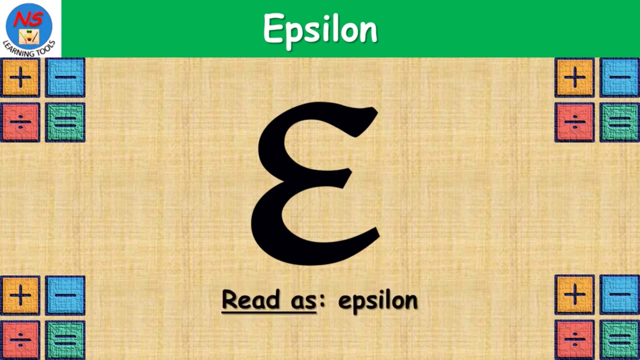 angle- read as angle. summation: read as sum of or sigma. braces: read as brackets. brackets: read as braces. parentheses: read as parentheses. epsilon: read as epsilon. division. slash: read as division. 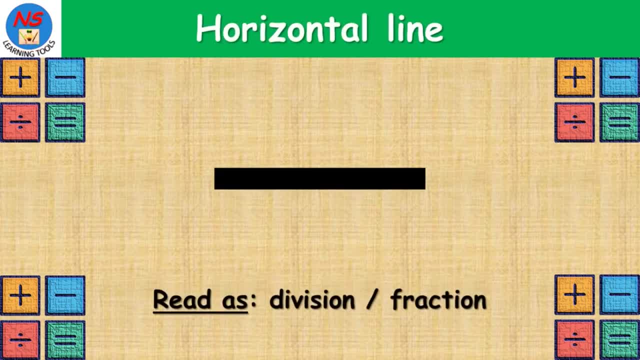 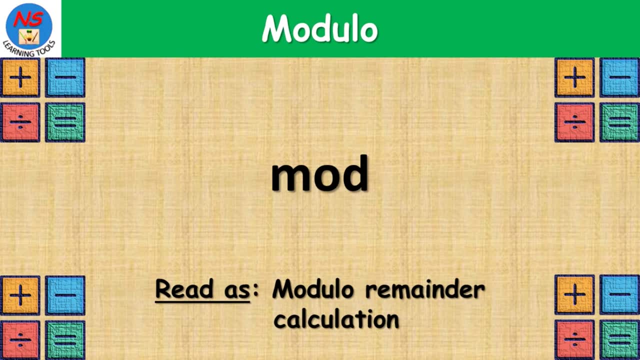 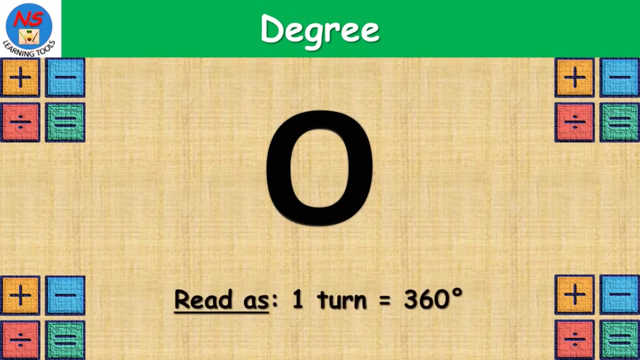 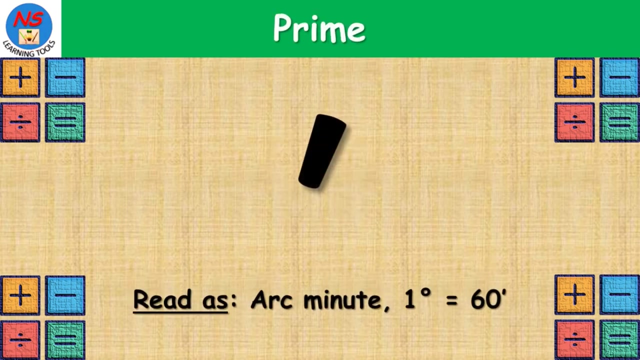 horizontal line: read as division or fraction. modulo read as modulo remainder. calculation degree: read as one turn equals to 360 degree. prime read as arc minute: one degree equals to 60 minutes. 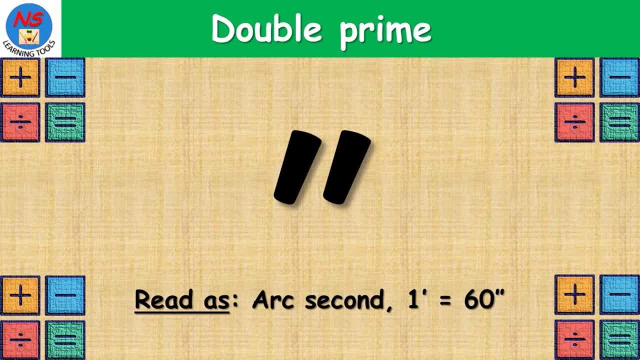 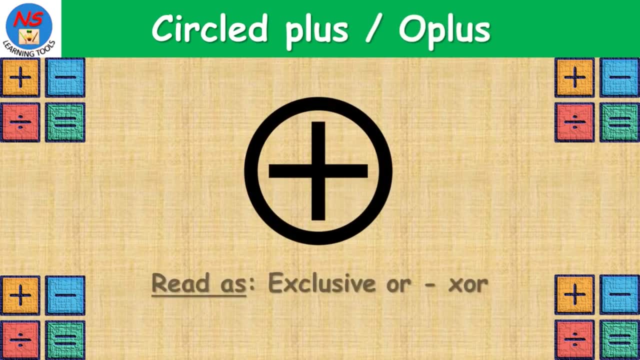 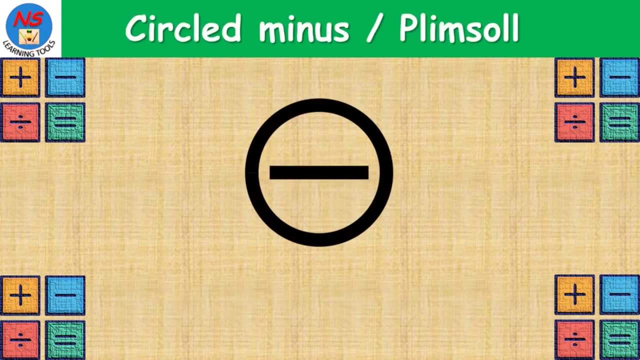 double prime read as arc second: one minute equals to 60 seconds circled plus or a plus read as exclusive or x or Circled Minus or Plimsoll Ritas Unicode Character. 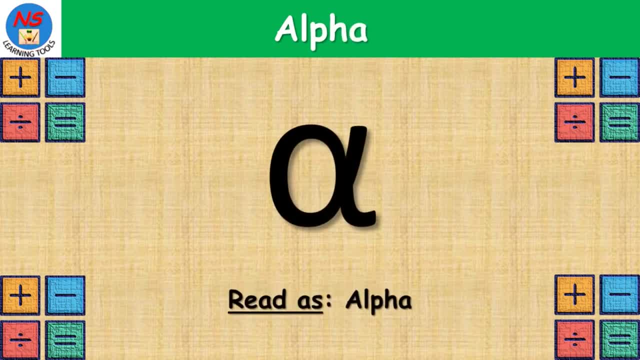 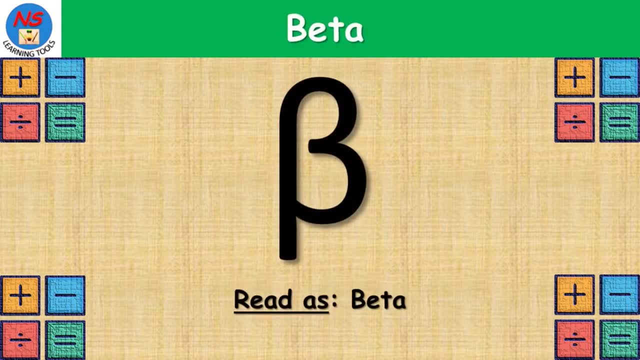 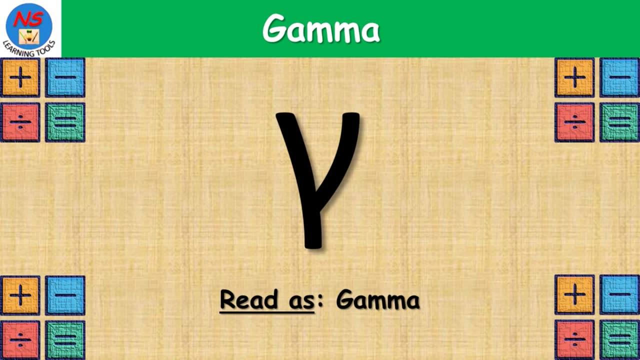 Alpha Ritas, Alpha, Beta Ritas, Beta, Gamma, Ritas, Gamma Lambda, Ritas, Lambda, Delta, Ritas, Delta. Asterisk, Ritas, Asterisk, Zeta, Ritas, Zeta. 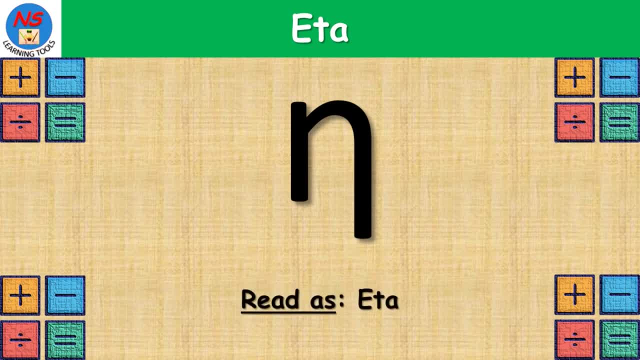 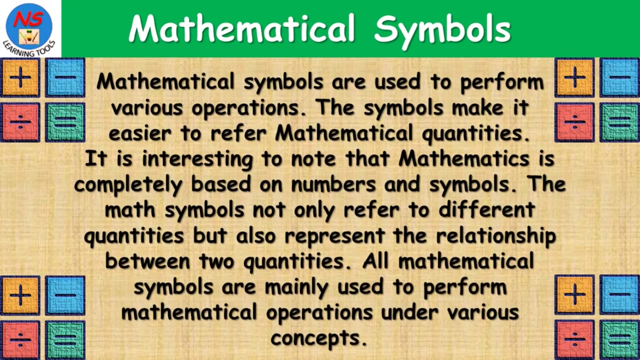 ETA, Ritas, ETA, Rho, Ritas, Rho, Ritas, Rho, Tau, Ritas, Tau, Sigma, Ritas, Sigma. Mathematical symbols are used to perform various operations. The symbols make it easier to refer mathematical quantities.